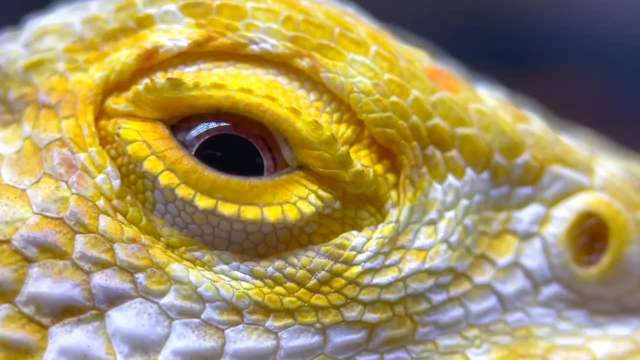 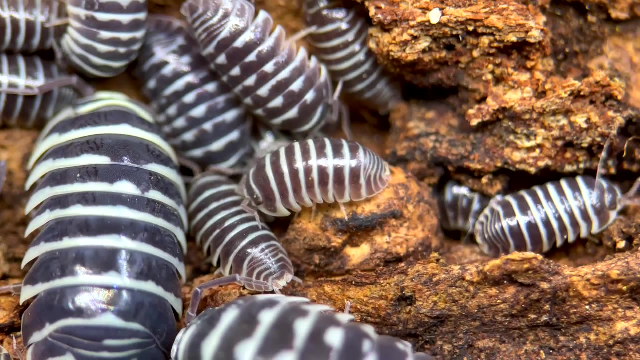 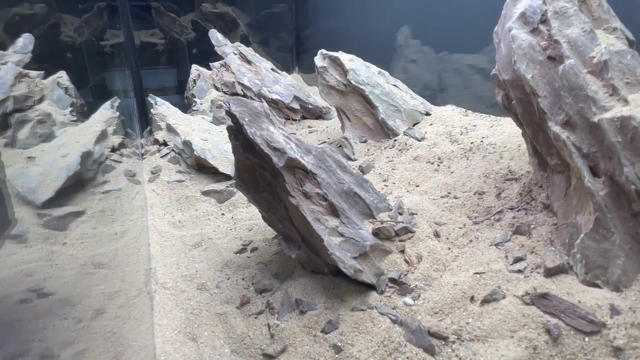 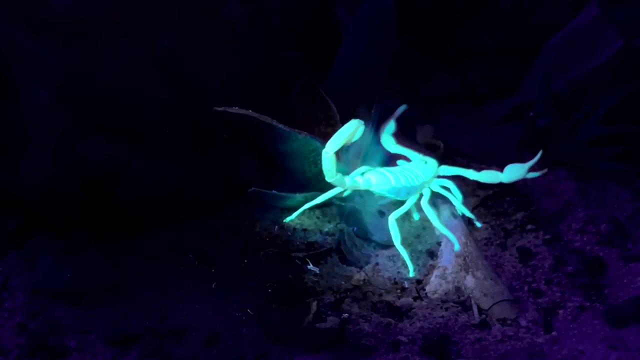 Within this tank lives a miniature world. There are predators and prey, wind and rain. This desert is a dangerous place, but despite all odds, some animals have evolved to survive. It transformed from an empty wasteland to a thriving ecosystem. To understand the mysteries within, first we must go back to day one. 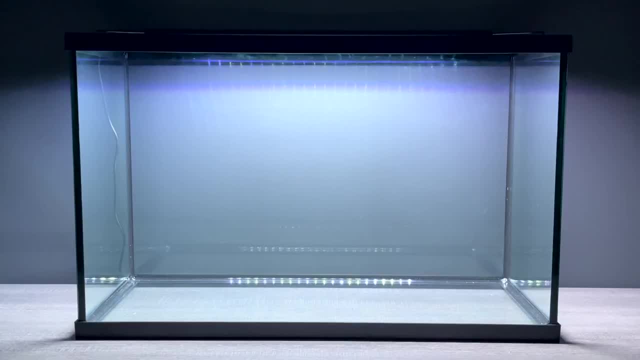 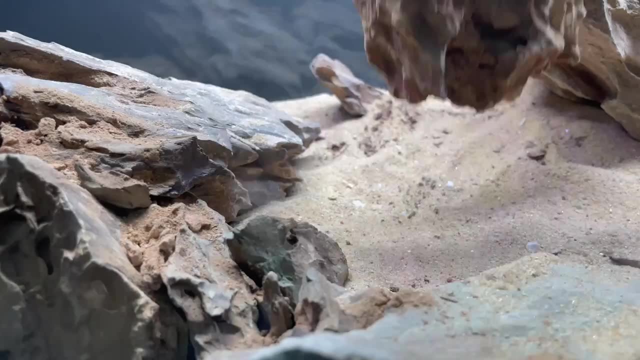 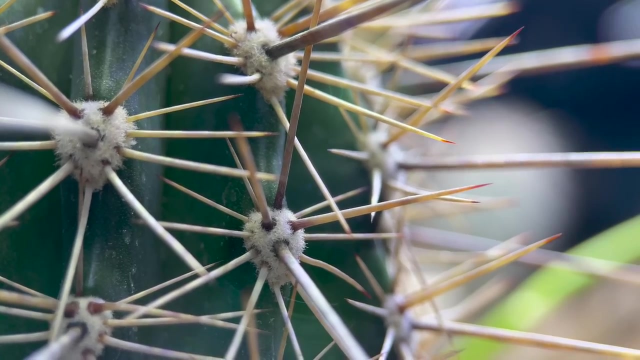 It all started when I got the tank, some materials and a whole lot of cacti. I proceeded to mix up some dirt and then build up the substrate. After placing in some rock, I began to plant the cacti. Their spines are extremely sharp and it was a huge pain to plant anything. 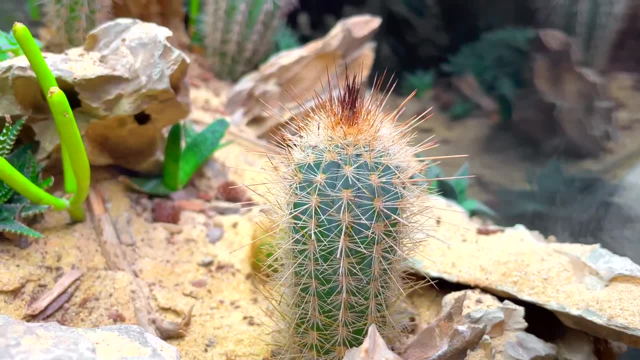 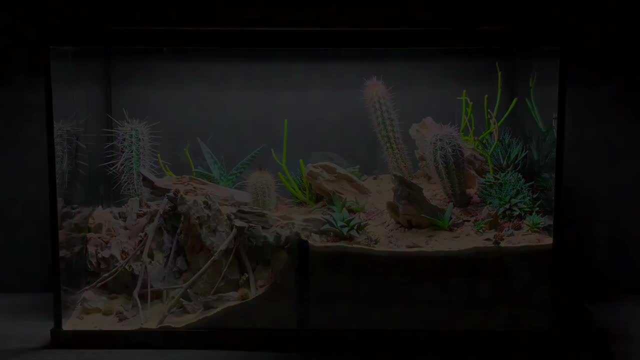 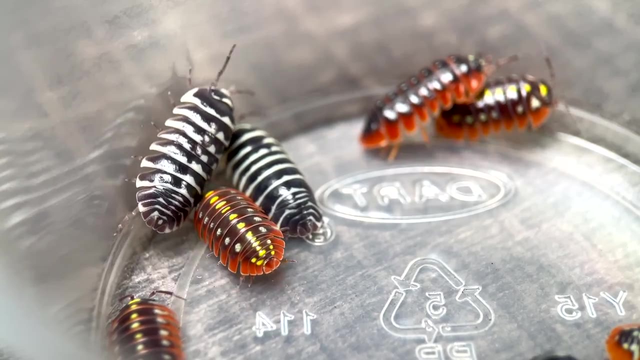 I added in some final touches and the tank was complete. This will serve as the foundation for a thriving ecosystem. On day three, I introduced the first animals. These are called isopods. As you can see, I have two varieties here: clowns and zebras. 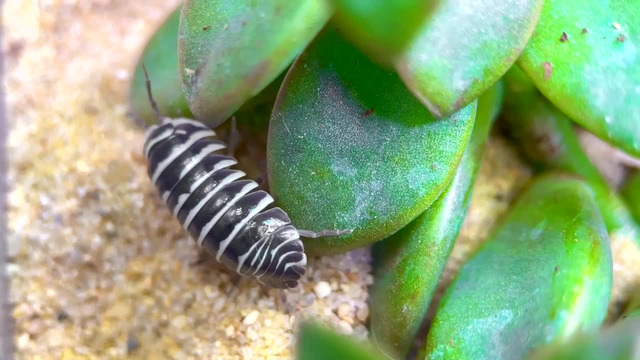 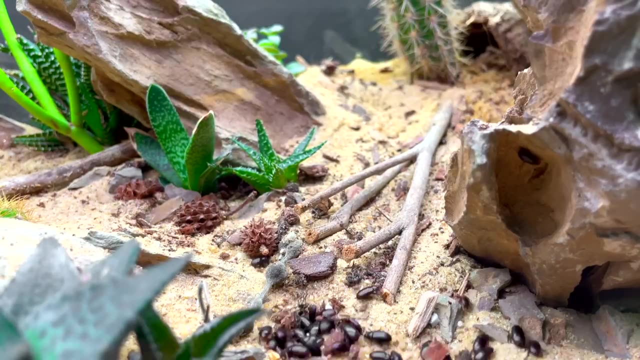 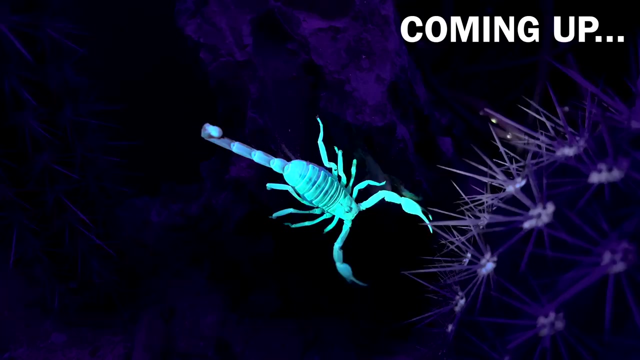 After I placed them in, they began to search for shelter. Alongside the isopods, I introduced springtails and buffalo beetles. These two detrivores will eat pretty much anything they can find. All of these tiny bugs will eventually be food for a future predator. 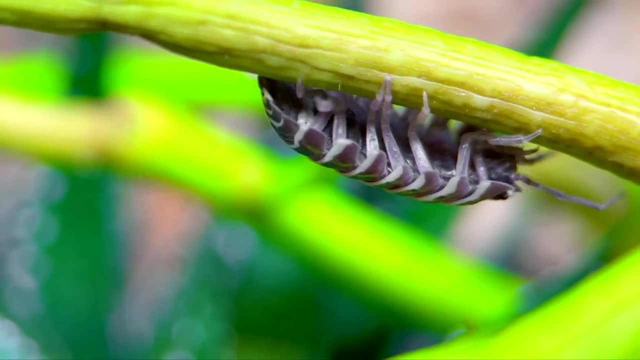 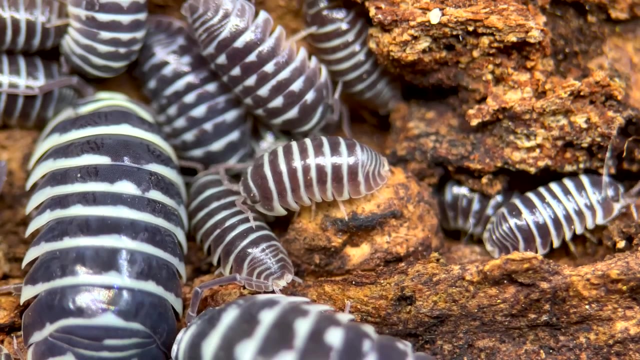 By day 50, the isopod population began to boom. In the shaded areas of the tank they would form small little herds. The juveniles looked almost identical to their adult counterpart. Here you can even see one shedding its skin. 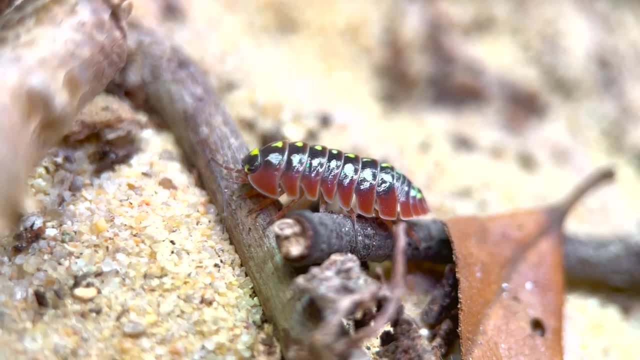 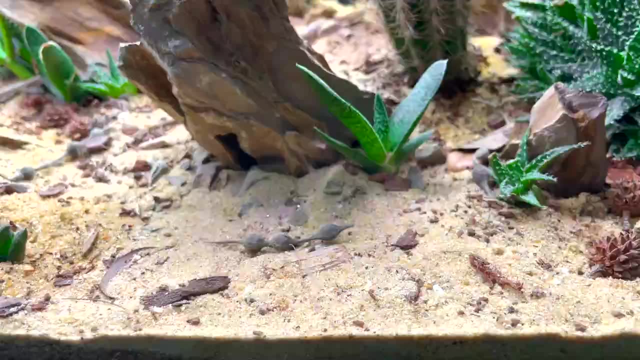 While the zebras were thriving, the clowns seemed to have disappeared entirely. On the other hand, the buffalo beetles were taking over. I placed a dead zebra. I placed a dead cockroach into the tank to show just how many there were. 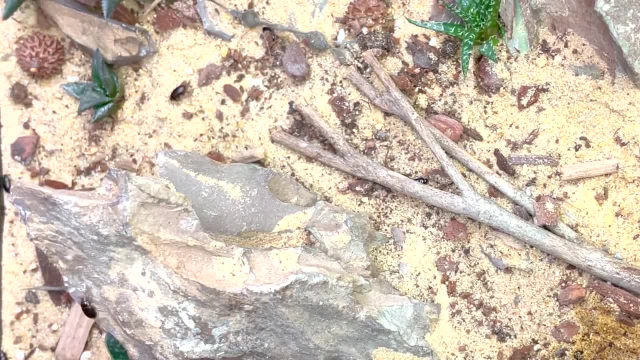 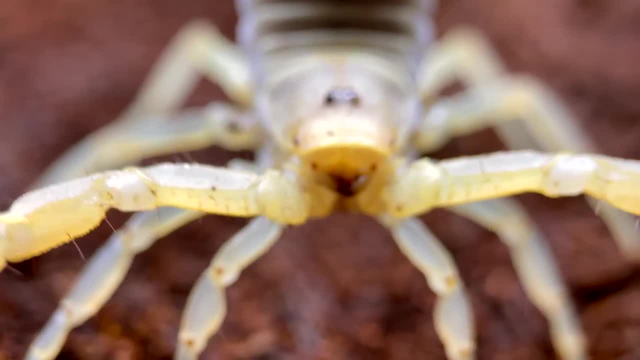 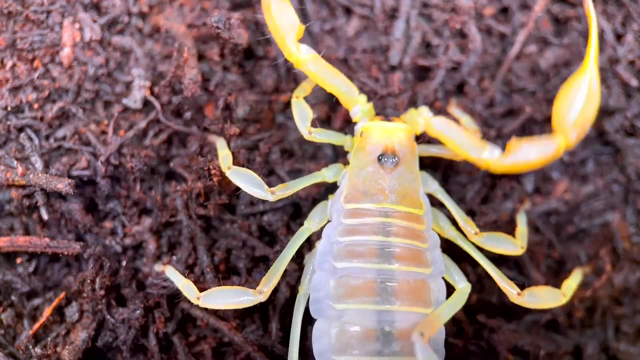 Soon, there was nothing left but a hollow skeleton. They were running rampant and I needed a predator. I needed something deadly, something fast, something almost as terrifying as my mother-in-law. Let me introduce you to the dune scorpion. He is a vicious predator and will make short work of a beetle or isopod. 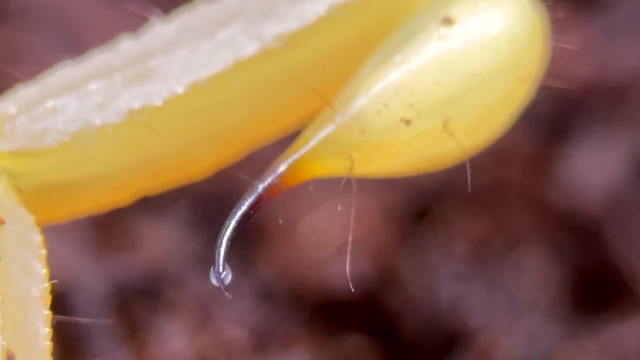 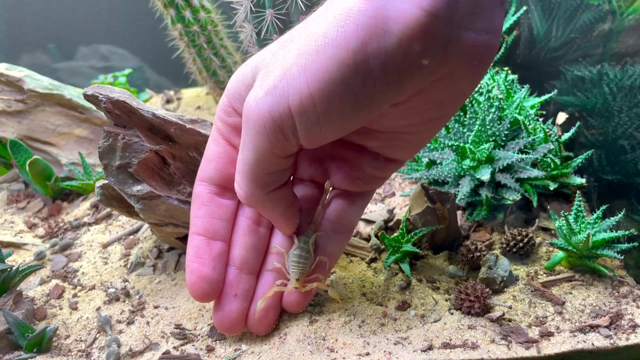 Do you see that tiny white drop on his stinger? Well, that is a potent venom and I have to be extremely careful. I picked him up and prepared to place him into the tank. After a gentle love tap, he took his very first step into the new world. 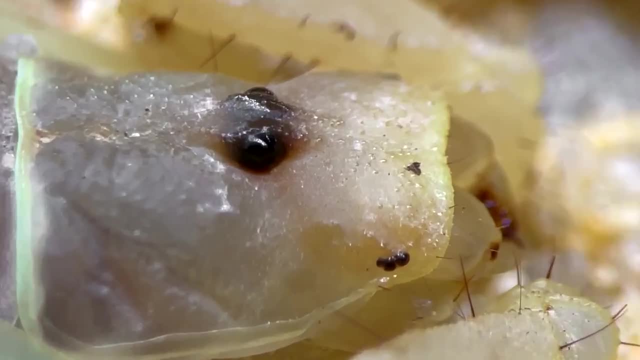 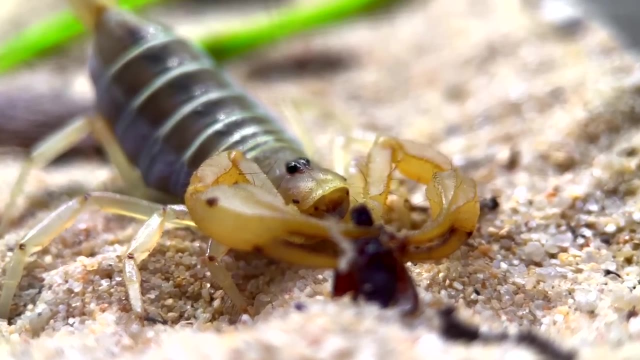 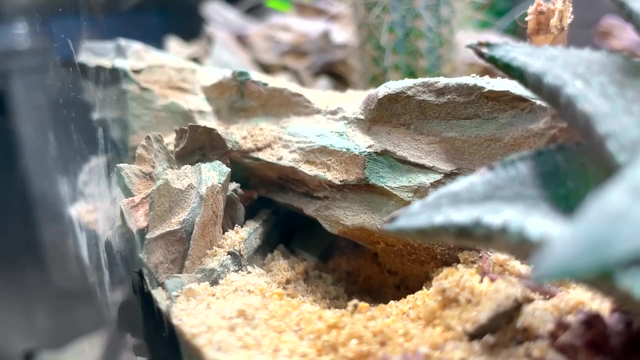 Scorpions are almost completely blind, so they don't use their eyes to get around. Within just a few minutes he managed to take down a buffalo beetle With a full stomach. he began to search for a place to burrow. After a few hours his burrow was complete and it just looked like an ordinary hole. 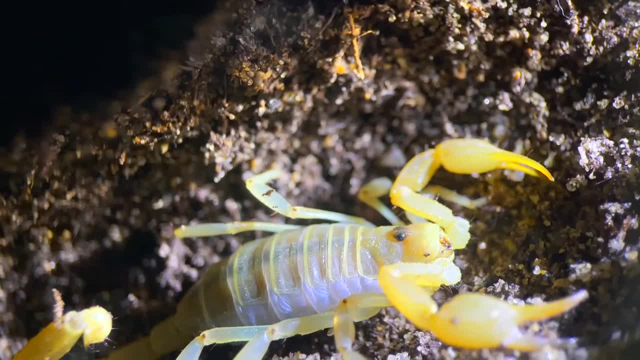 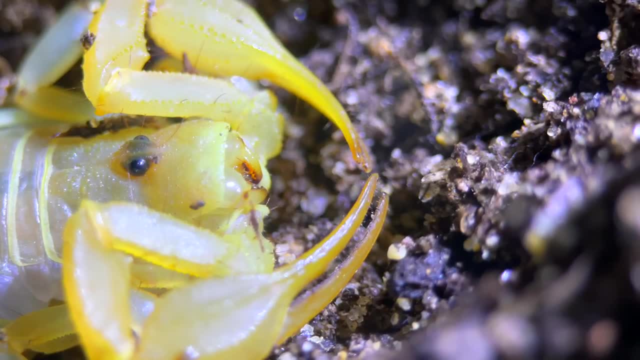 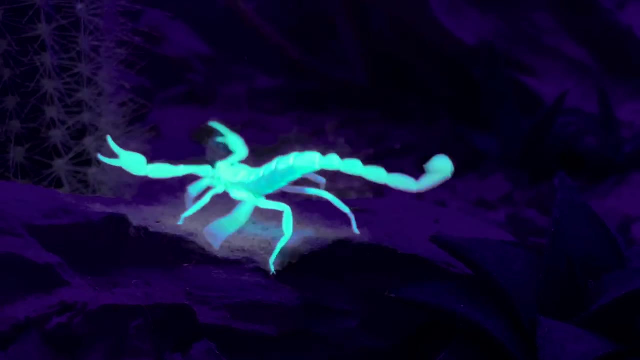 But if we look underground we can see it is so much more. It is his home. He would spend most of his time here, but as day turned to night he would emerge Under ultraviolet light. he will glow a radioactive green. 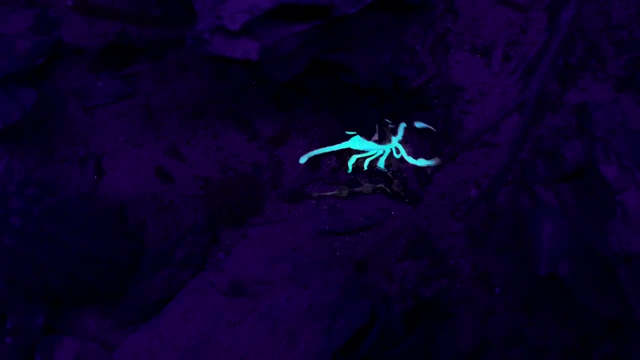 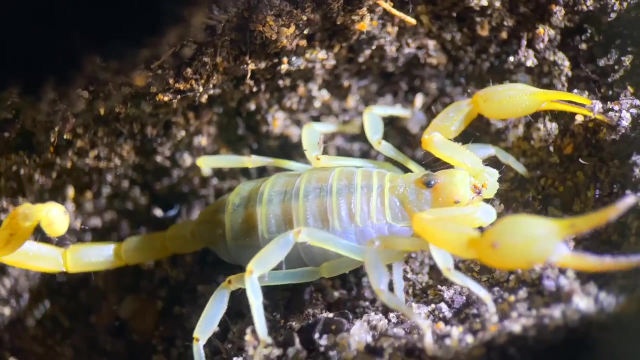 He will be a perfect enemy for the future. He will be the most beautiful human being in the world. On day 60, I realized the scorpion wasn't going to be enough. The beetles were breeding faster than the scorpion could eat them. 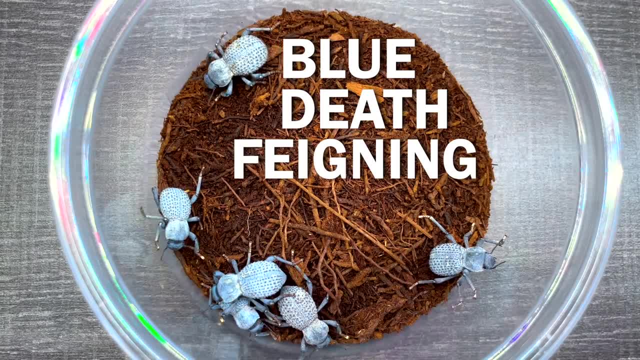 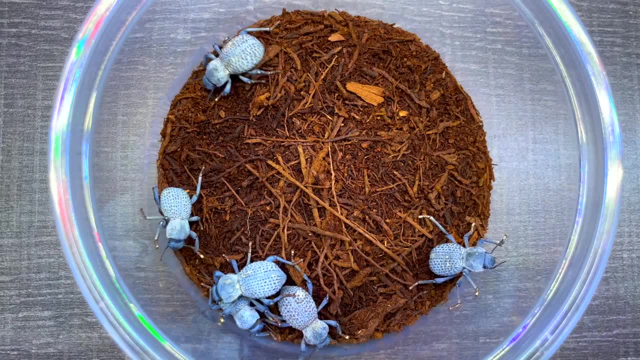 I needed to add competition. Meet the blue death fainting beetle. This is no ordinary bug. They have three superpowers. First off, they make their own sunscreen. This white powder on their shell will protect them from the three deadly bugs that they are fighting. They are the first to be killed by the scorpion, But they will be killed by the blue death fainting beetle. This is the last of their powers. This white powder on their shell will protect them from the scorpion. They are the only ones that will survive. 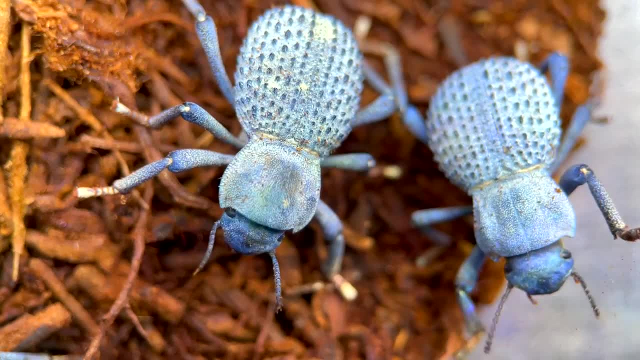 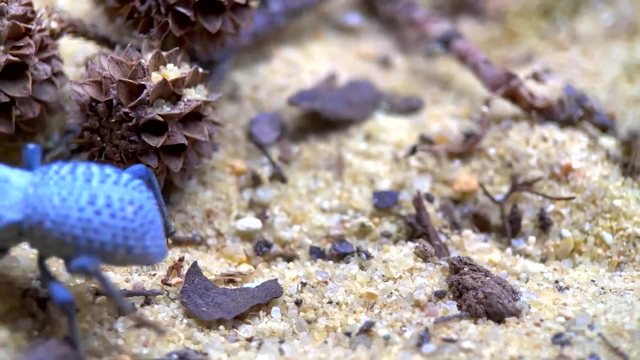 They will be the first to survive. They will be the first to survive. shell will protect them from the desert sun. Secondly, they have a huge abdomen to store water, kind of like a camel. they can last for ages without any water at all. 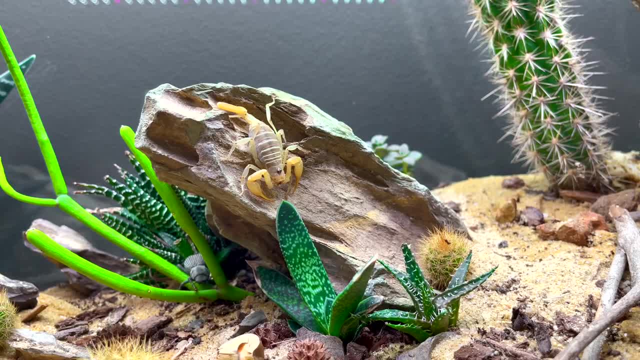 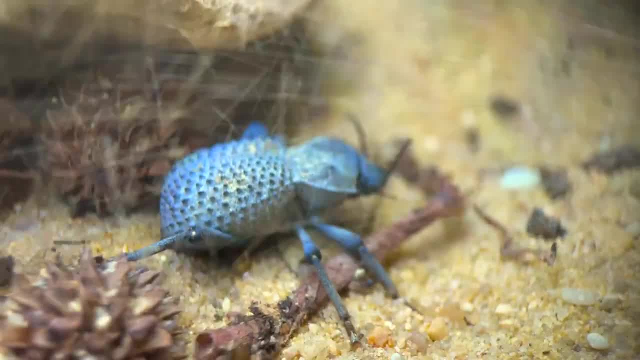 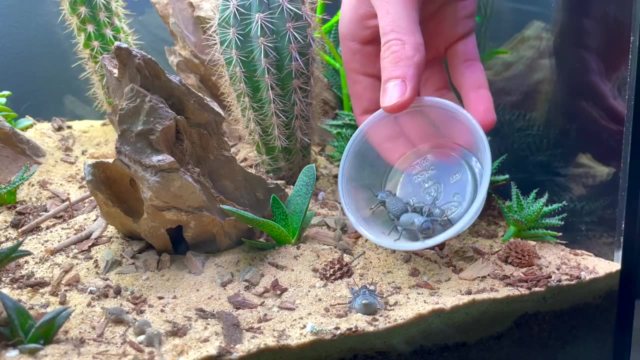 But if a predator tries to eat them, that's where its third superpower comes into play: They are indestructible. Their thick armor will protect them from sandstorms and strong desert winds. I added them into the tank and immediately one was making a fatal mistake. 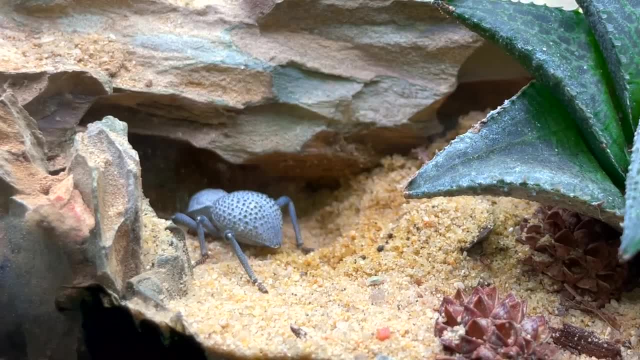 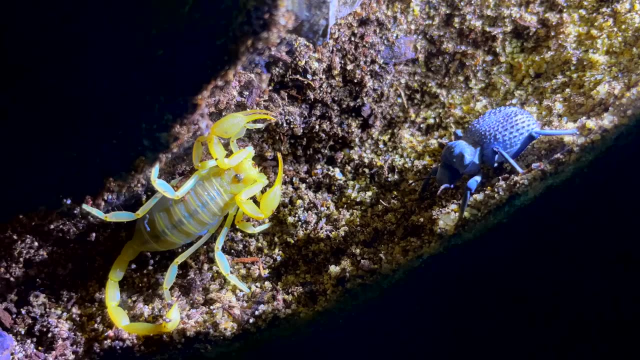 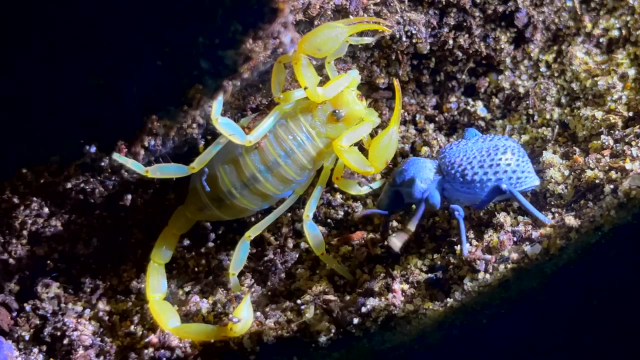 He wandered towards the scorpion burrow and then down inside. He was walking towards his doom. There was a stalemate. The beetle made his move, He tapped the scorpion and then retreated deeper into his burrow. The scorpion gave up. 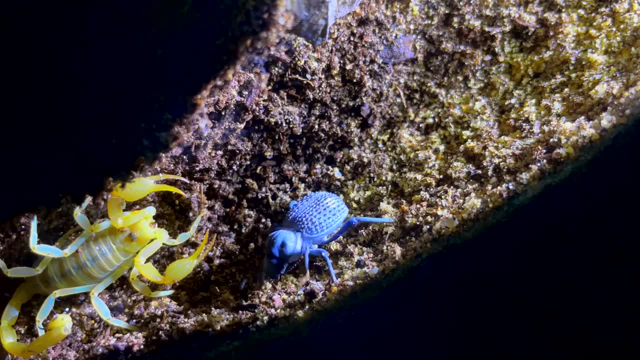 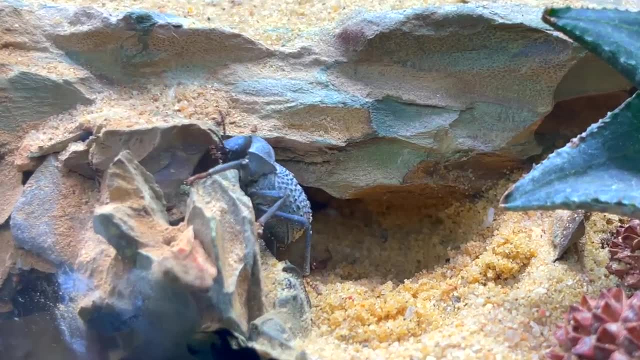 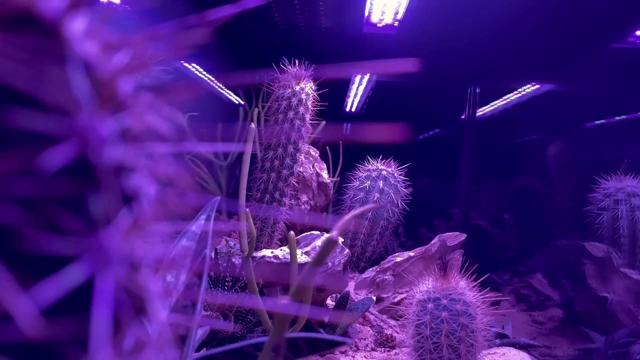 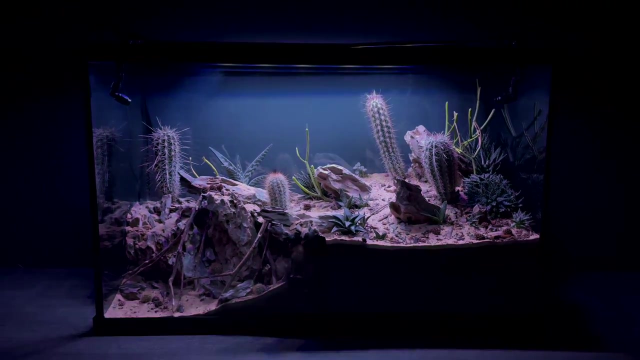 He gave the beetle a gentle push and then made his journey back to the surface. That was a close call. I decided to let them be overnight As the sun began to rise. something extremely rare was about to happen: It was rainy season and one of the few storms of the entire year was about to commence. 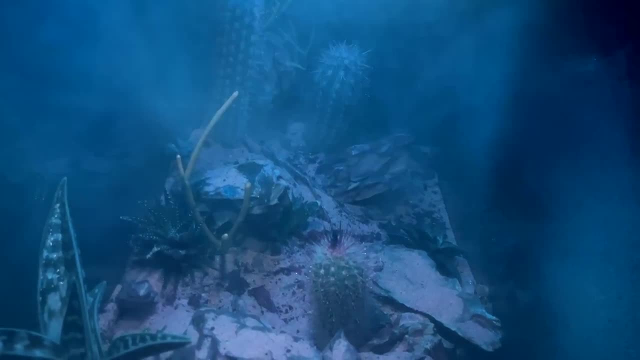 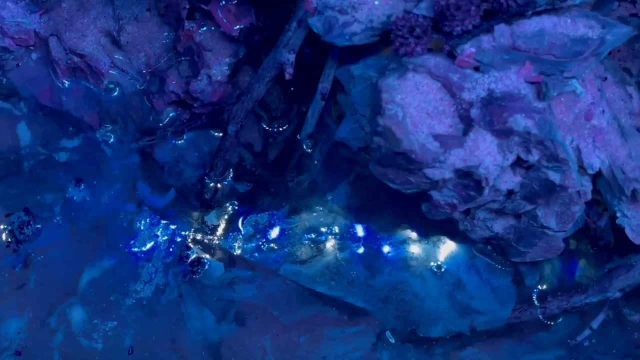 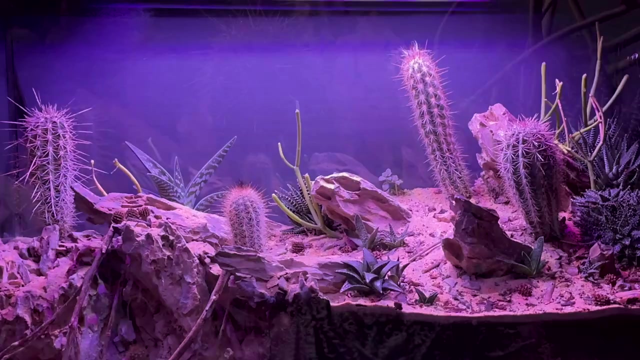 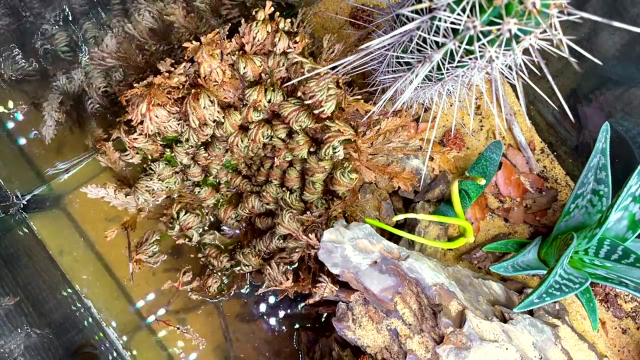 The tank began to flood. As the storm faded away, animals began to emerge. The rain brought new life to the desert landscape. This rose of Jericho opened its leaves after receiving water. The rain was so heavy that it was hard to breathe. 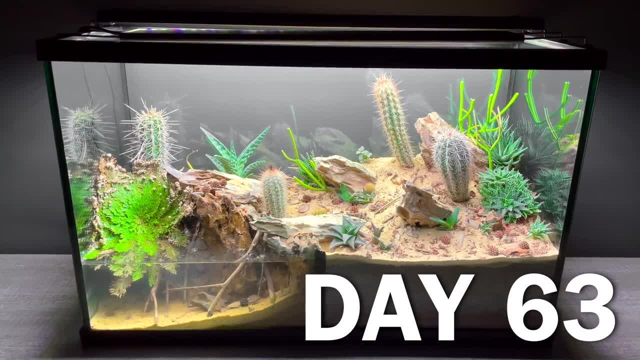 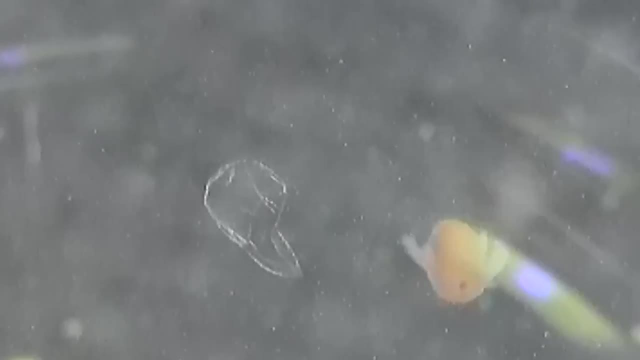 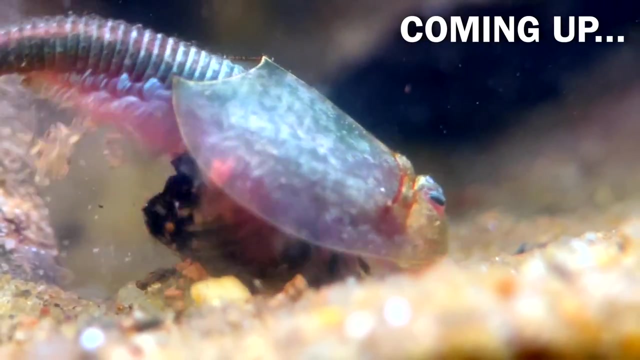 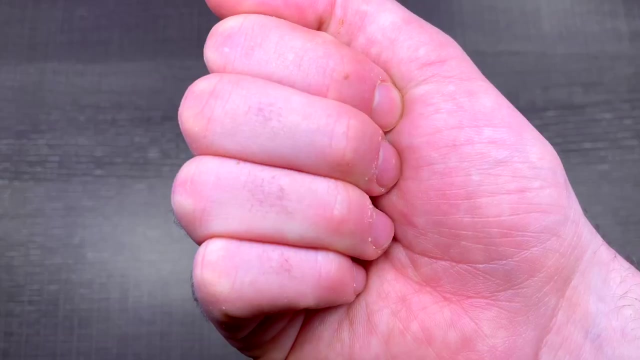 Hundreds of tiny eggs that laid dormant in the sand began to hatch. The pond was swarming with these tiny white dots that were going to become something incredible. Meanwhile, on land, I figured it was time to introduce a new animal. Here is a Mexican jumping bean. 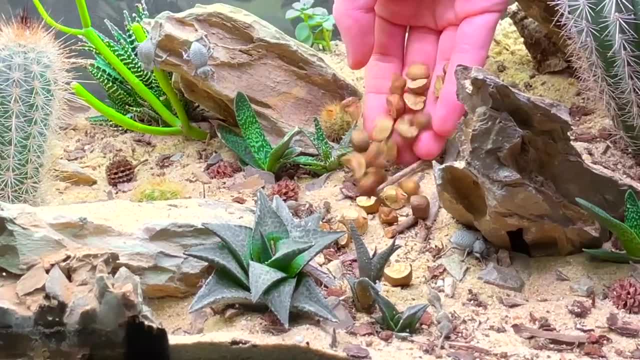 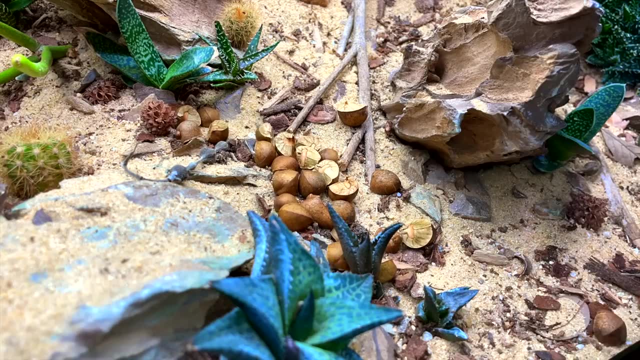 And here are 30 more. These are not what they seem. After I added them in, they began to dance. They seem to roll around mindlessly, but each one is on a mission: Find shelter. They jump to escape the desert heat. 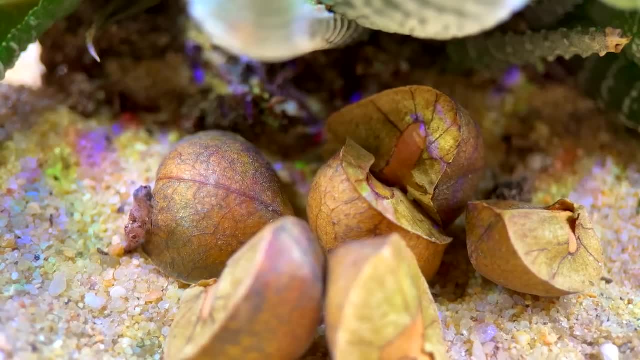 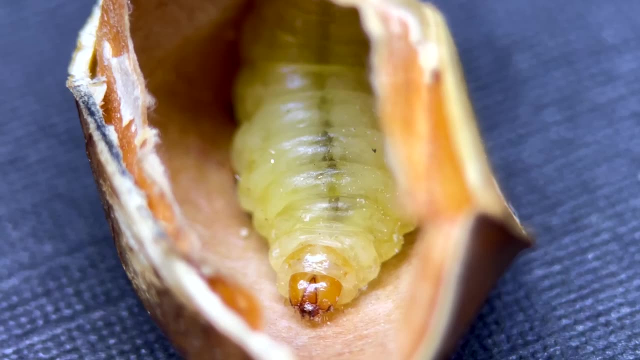 It didn't take long for them to huddle under whatever they could find. Now, inside every being lives a caterpillar. One day they will emerge into a beautiful little moth. By day 72, life in the water had grown substantially.